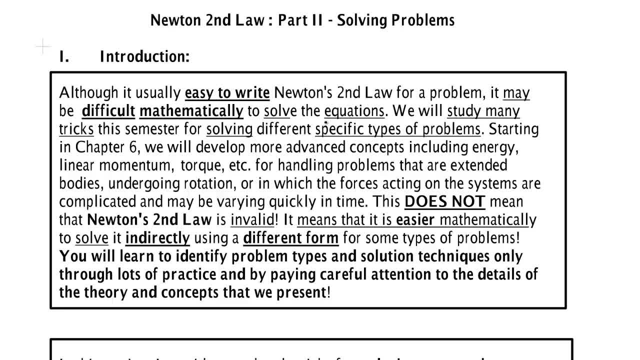 We will find out in later chapters that when Newton's Law is very difficult to solve, new concepts like energy, linear momentum and angular momentum can be developed, which will help us solve problems. This doesn't mean that Newton's Law is invalid in situations where we apply this concept. It simply means that the equation may be difficult to solve and by using these other concepts we can get to simpler equations. 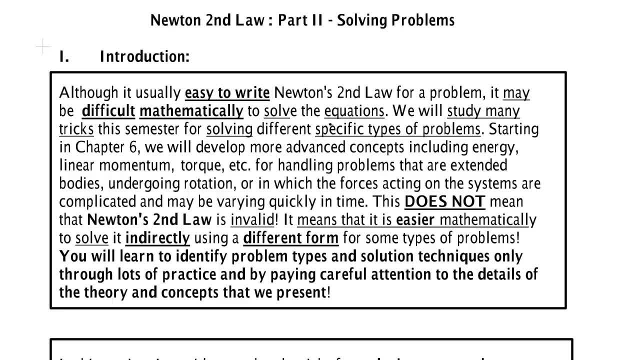 In general. for all the problems we will be looking at in this course, Newton's Second Law is true. It is just that it may be difficult to solve. The first such type of problem where you can get a trick that I can help you solve Newton's Law are incline plane problems. 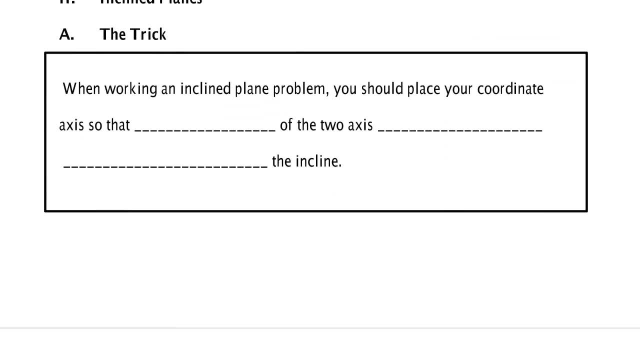 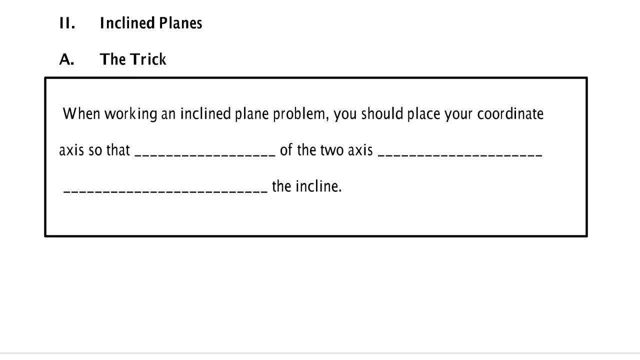 So let's look at some incline plane problems. The incline plane problem could be solved in many ways, but the trick to make the math easier is that when you work an incline plane problem you should place the coordinate axis so that one of the two coordinate axes 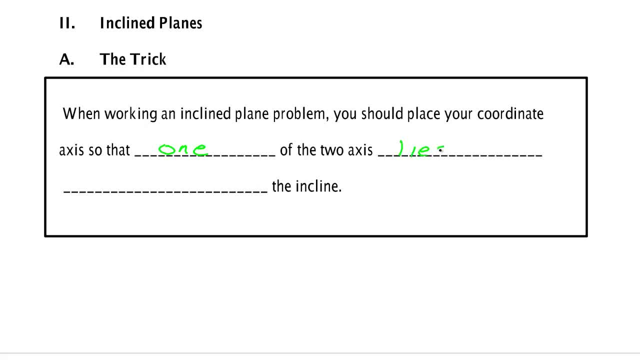 lies along the incline. In other words, you should rotate your coordinate axis. Now this may seem like an unnecessary thing to do- and I didn't say that you can't solve incline plane problems without doing this- but it will make the math a whole lot easier to work if you do this trick. 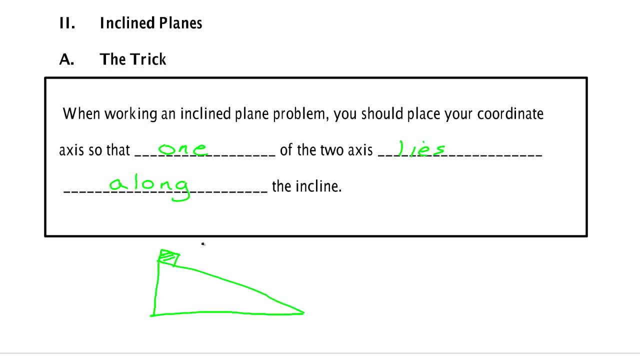 So let me show you. All you have to do is that when you run into an incline plane problem, you should rotate your coordinate axis. When you run into an incline plane problem, lie your axis with the x-line along the plane and the y-axis perpendicular to this. 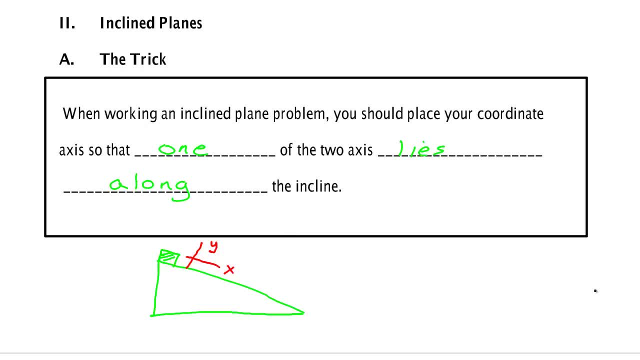 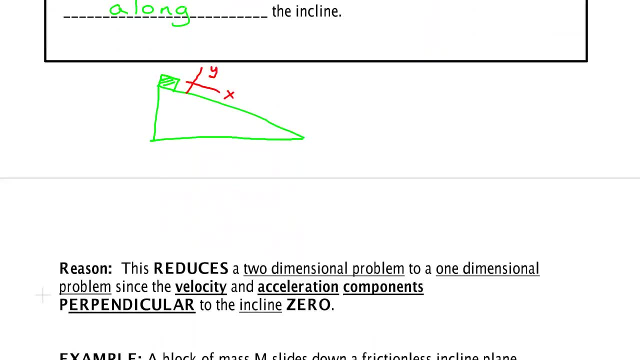 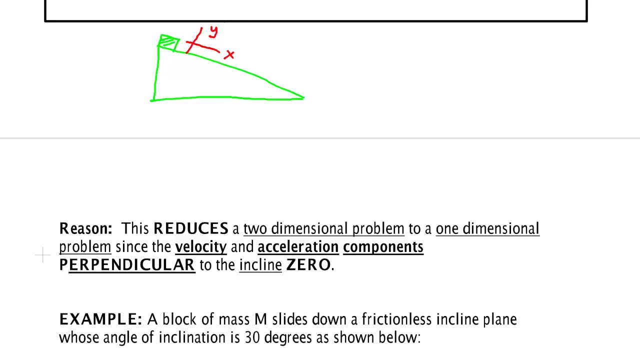 That's it, And the math will be much simpler in solving the equations. Why is this? Well, it turns out it's a relatively simple thing to understand why it is. When you do this, you take a two-dimensional problem where the object could be moving in two dimensions had you put your axis, as in the blue case. 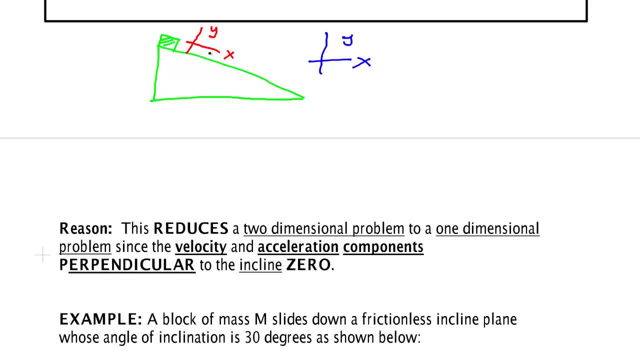 Let's say like this: So as this block moves this way, he moves both along x and y if you use the blue axis, But if you use the red tilted axis, as he moves along this direction, he's moving along x. He has no motion in y, so he has no velocity in y. 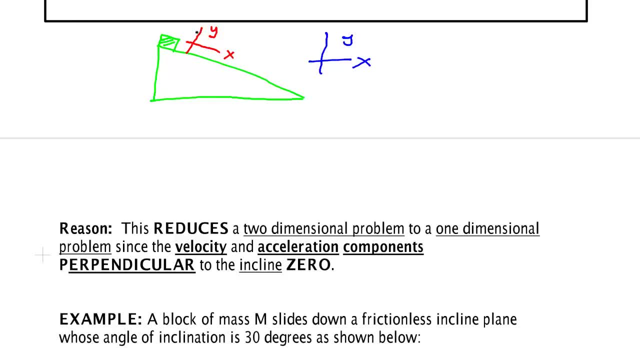 Furthermore, the velocity in that direction isn't changing, so he has no acceleration in that direction either. This makes those set of equations for the y-direction very simple. So the whole reason is that it reduces a two-dimensional problem to a simpler one-dimensional problem, since the velocity and angular acceleration components perpendicular to the incline are lost- a word here- are zero. 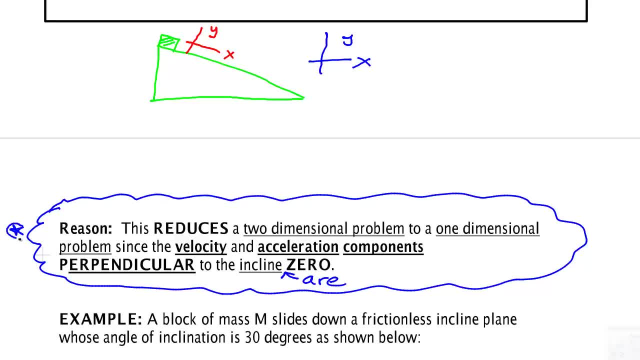 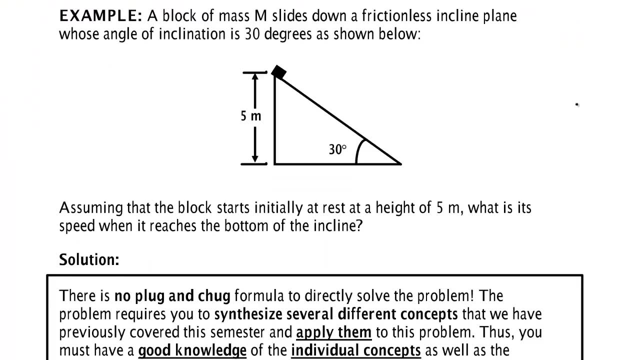 So that's the whole reason why the trick works. You just need to do the trick whenever you have it occur. Now let's show you this trick being applied. Here's an example problem: You have a block of mass m sliding down a frictionless inclined plane whose angle of inclination is 30 degrees. 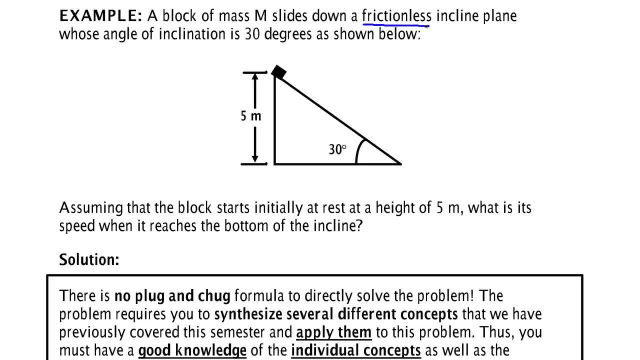 Important things to note is it's a frictionless inclined plane. There'll be no friction in this problem. It has an angle of inclination. It's 30 degrees. We're going to assume the block starts initially at rest. It's at a height of 5 meters. 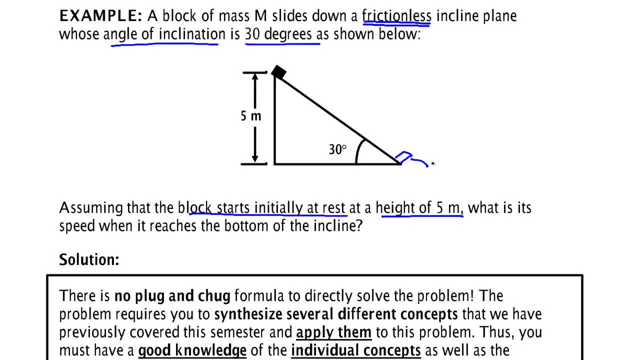 We're going to want to know how fast it's going when it gets right down to here. So for this problem, I'm going to lie my x-axis along the plane and I'm going to know that up here vx-naught is 0 meters per second. 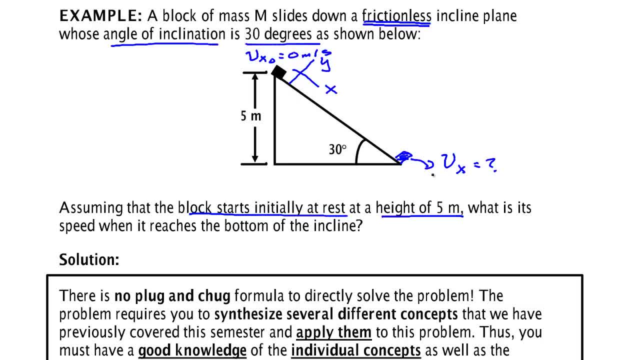 and sometime later down here it's going at some speed. This distance, which I'll call x, is the length of this incline. So this guy right here is x equals 0. This distance all the way down, which is the hypotenuse of this triangle, is L. 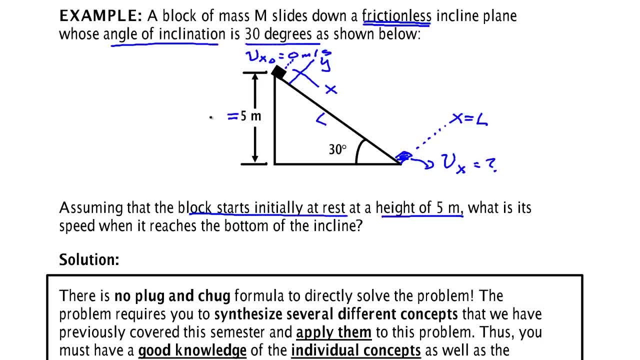 So that's L, And I'll give this symbol the symbol H. Now, there are no plug-and-chug formulas. You're not going to look in the book somewhere and find a formula that says for inclined plane. this is how the formula that you get for this. 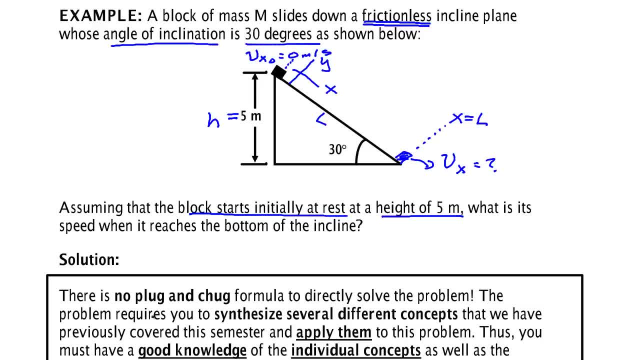 You're going to look for the speed of the block. The whole reason for doing these problems isn't just to learn physics. It's to learn how to solve problems, And solving problems are useful for your career. They're useful for your future academic. 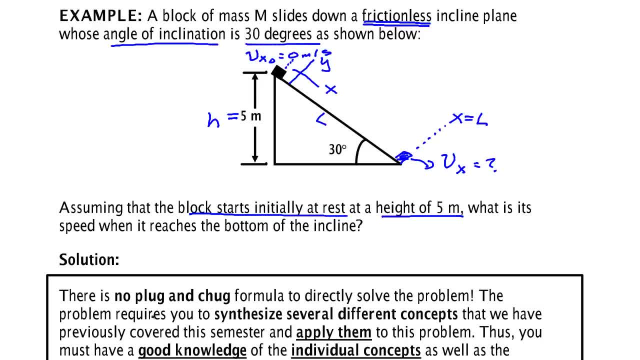 What you have to do is take ideas that we've already covered and put them together like pieces of a jigsaw puzzle or like moves in a chess game, in order to build something pretty brilliant out of this to solve this problem. These require higher reasoning. 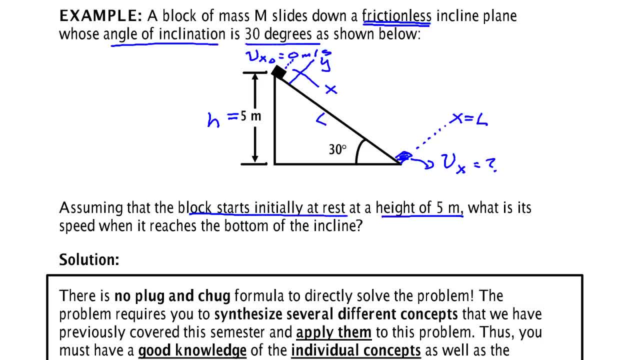 And this is one of the reasons that you're in a physics class- is to build these reasoning skills. So I've aligned my axis like this: I look at the problem and say, hey, I don't have any basic formulas for solving the speed. 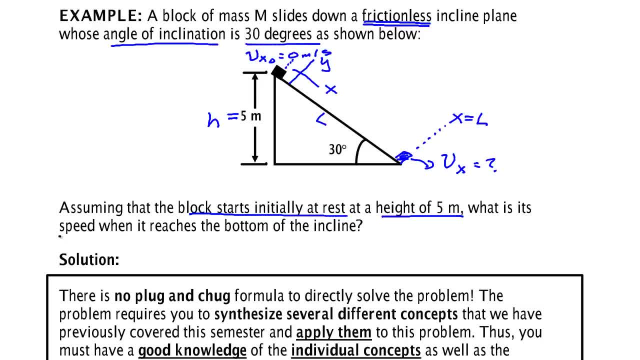 when it reaches the bottom of an incline. What physics do I know? Well, I wasn't given an acceleration time graph, so I can't just find the area under the curve. to find the change in velocity, The kinematic equations might be very useful. 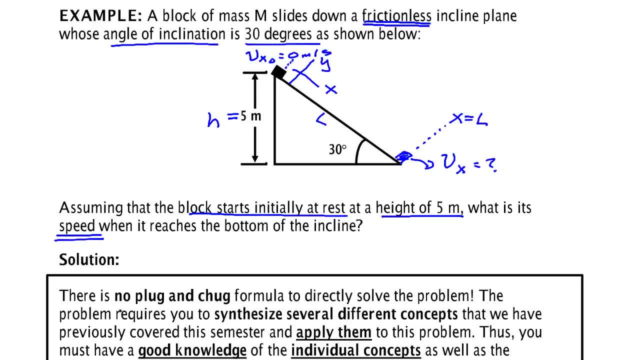 but I'd have to know the acceleration, and I'd have to know that the acceleration was constant. And I'm not given the acceleration in this problem. So what I do know- that's always true- is Newton's Law. So let's apply Newton's Law to try to solve this problem. 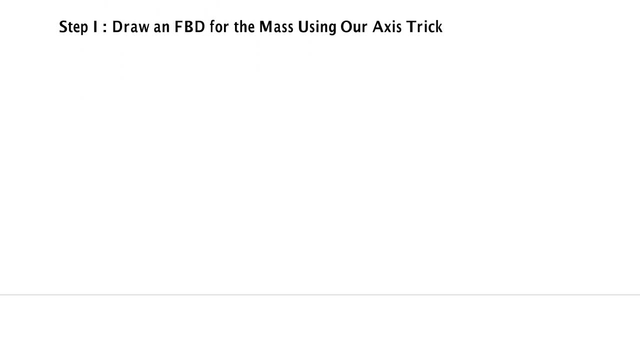 So if I'm going to use Newton's Law, I'm going to draw a free body diagram. So first thing up here I'm going to draw my free body diagram. There's my isolate the body. Second, I apply want f to find the weight. 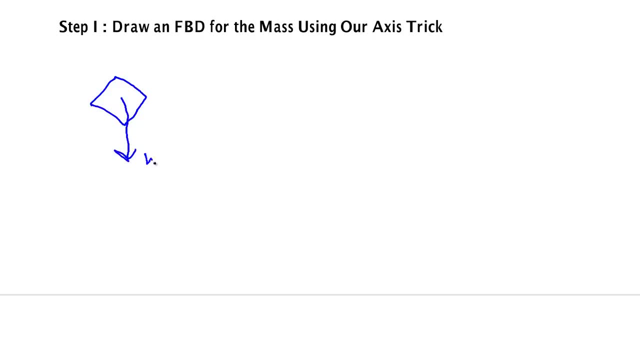 Weight points straight down. Not a very good drawing. Hopefully you can do better than I can with my pen here. Applied or no? applied Is there a normal? Yeah, a normal applies the force from the incline upon the block. Are there any tensions? 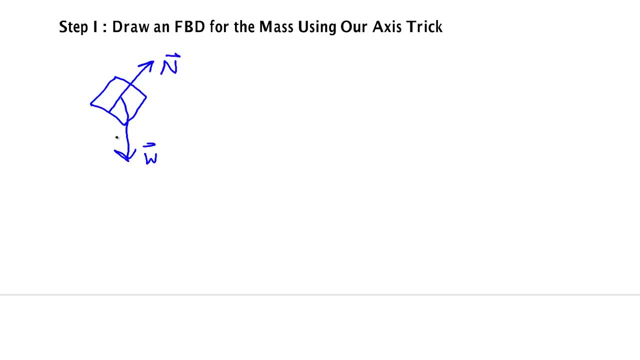 No, there's no tension Friction. No, there's no friction. So that's all the forces. This angle here is theta, And we said that we're going to make our axis x and y. So that's my incline. free body diagram for the mass of the inclined plane. 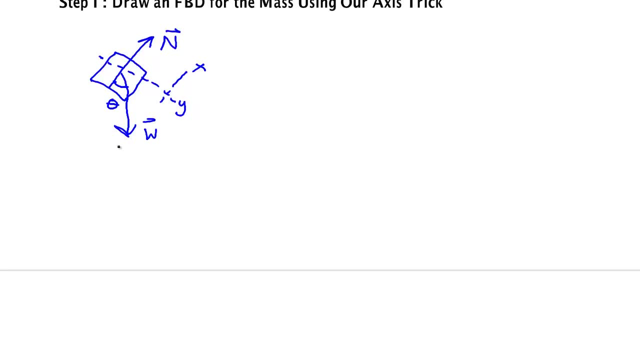 Now I'm going to use this free body diagram and read it in order to write Newton's Laws. So in writing Newton's Laws off my free body diagram. sum of the forces in x is mass times acceleration in x. Sum of the forces in y is mass times acceleration in y. 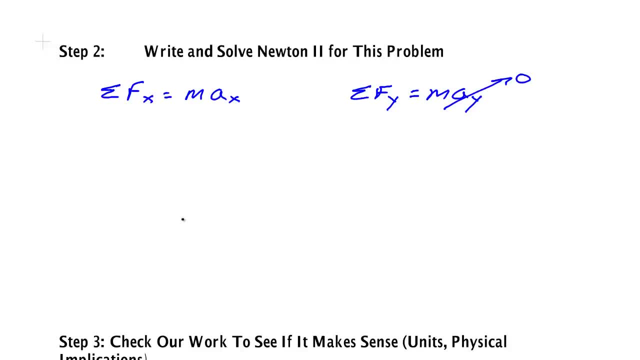 But we know there is no acceleration in y because of the way we put our axis In the x direction. the only vector pointing in the x direction is the weight. So I go back up here and I look and I say, hey, the only thing I have is this side of this vector. 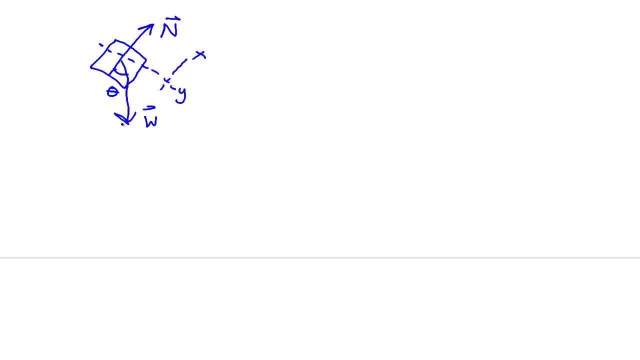 That's the opposite side. So that means I need the sine function And it's in the positive x direction. Oops, sorry, made a mistake here. This should be y and that was supposed to be x. It changes everything if I don't make it that way. 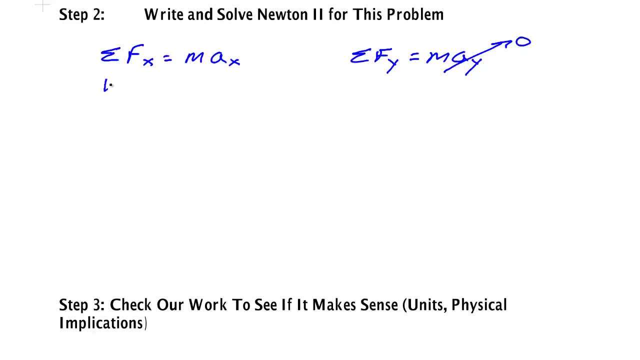 So down here I have w sine, theta is max, And over here for the y. going back up, all of this force is in the y direction And this side of the weight, which is the adjacent side, the cosine, is in the negative y direction. 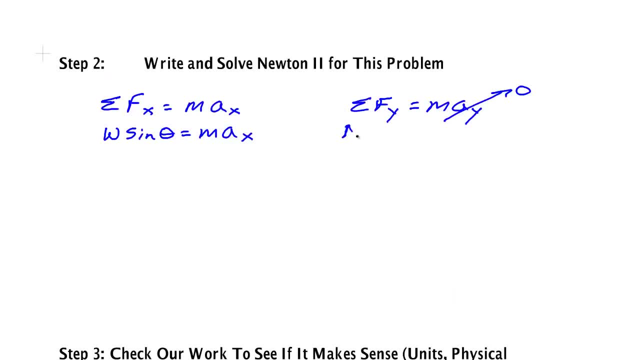 Alright, so I have normal minus w. cosine theta is zero, So the normal is equal to the weight, which is mg times the cosine of theta, And that's one fact that I know Don't really need it for this part of the problem. 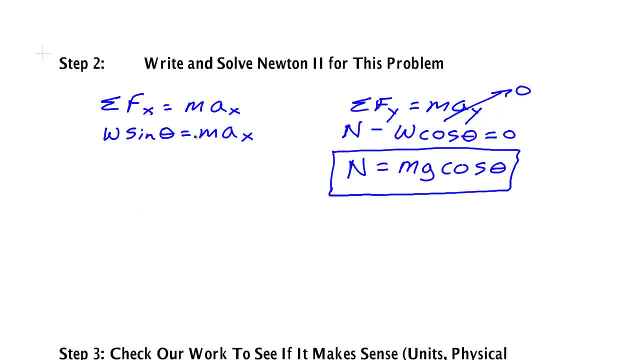 I need the normal when I'm dealing with friction problems Over here. weight is mg sine theta And that's equal to max, But I see that I don't need to know the mass. Ax is g sine theta. This shouldn't be surprising by now, that you don't need to know the mass to find the acceleration. 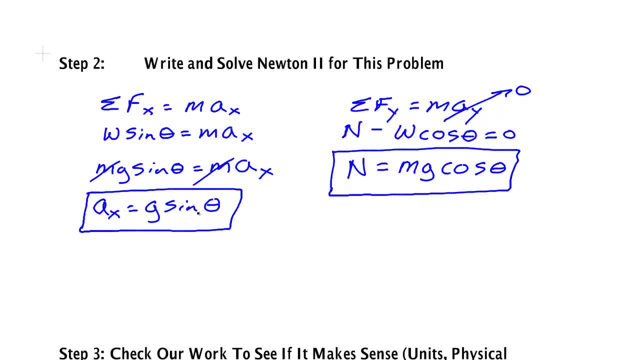 Because gravity means that this is the falling body. It's just not falling at g, It's falling at something less based on the sine theta. Now, once you get an equation, before you start doing anything with it, you need to check to make sure it makes sense. 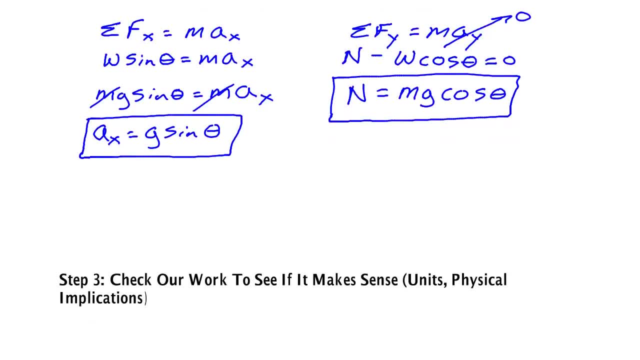 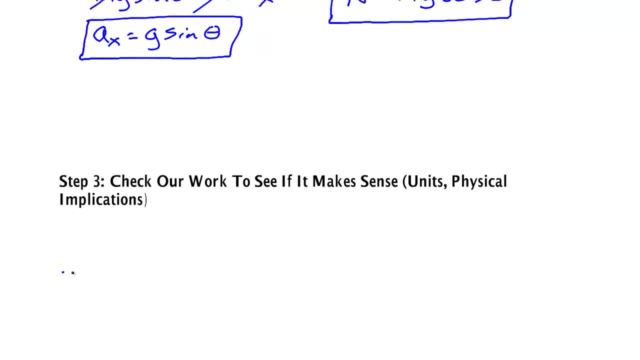 So let's check to see if this thing makes sense. Let's take a couple of extreme cases. One case would be if we made our incline plane flat, So theta was zero degrees. If it was a horizontal flat table, I know the acceleration would be zero. 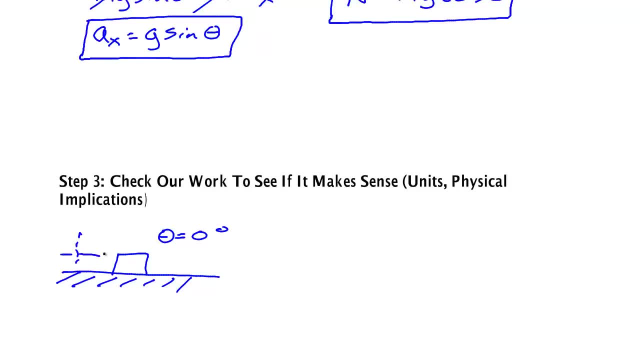 The block wouldn't want to move. The block would just stay where it is. Let's see if my formula gives me that Ax is equal to g times the sine of zero degrees. But the sine of zero is zero, So I get zero meters per second squared. 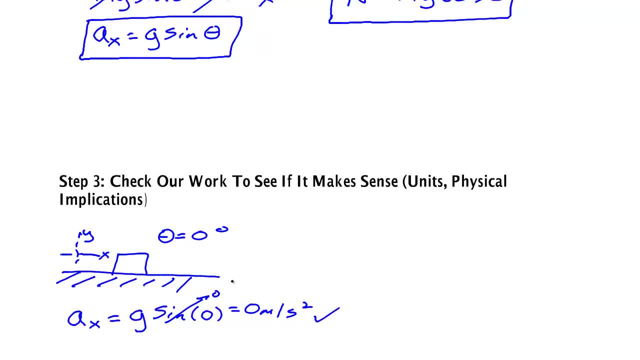 Check That makes sense. I want to look at the units of this plane, The units of this formula. The units of this formula are: g sine theta. Sine theta has no units. g has the units of acceleration, Ax has the units of acceleration. 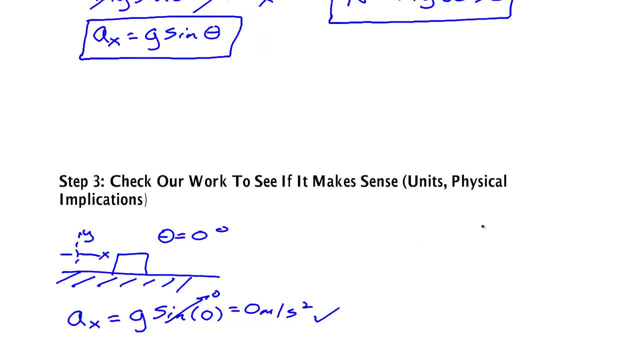 Units make sense. Let's try one more possibility. What about if I tilted my incline plane here? So theta was 90 degrees And here's my block. Well, in this case this block would have no other force except weight pulling it straight down in this direction. 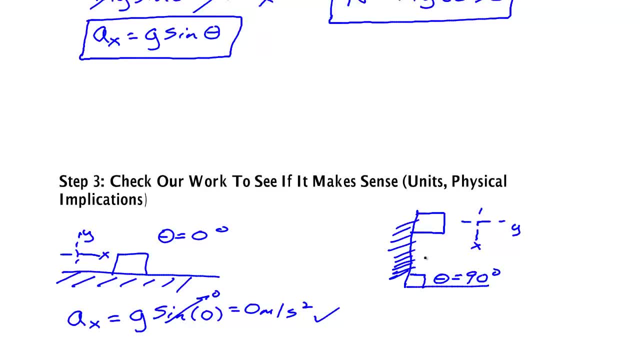 The normal would be like that. So the force would be g, I mean would be the weight, And the acceleration should be g. It should be a falling body. Let's see if that works out. Ax is g sine of 90 degrees. 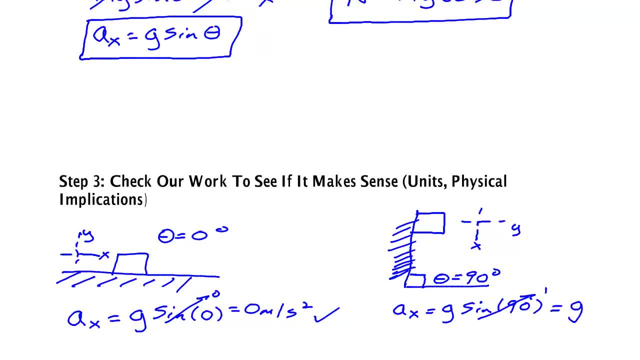 The sine of 90 degrees is one, And we just get g. So it makes sense. Our formula makes sense. Now it's more than just makes sense. We can see something else that's important: g is a constant. The theta is given to us as a constant in the problem.